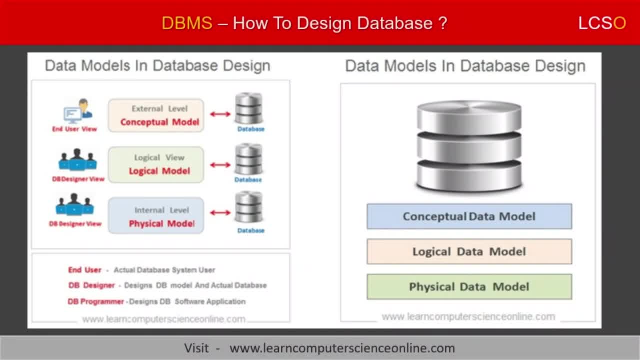 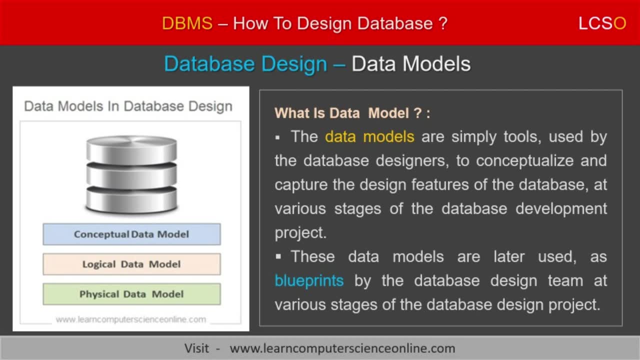 such as data model. The data models are simply tools used by the database designers to conceptualize and capture the design features of the database at various stages of the database development project. These data models are later used as blueprints by the database design team at various stages of the database design project. The database models make it very easy to visualize. 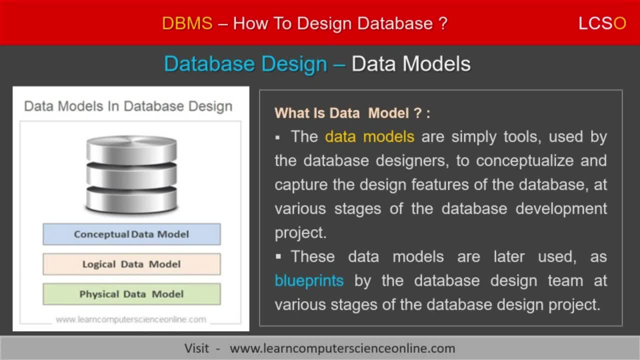 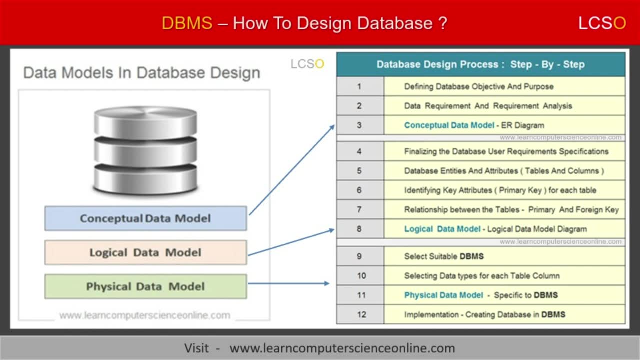 and communicate different design features of the database. All right, so now we are clear about what data models are and its purpose. Let us now move on to our main topic, that is, overview of the entire database planning and development process. The entire database planning and design process can be broadly split into two. 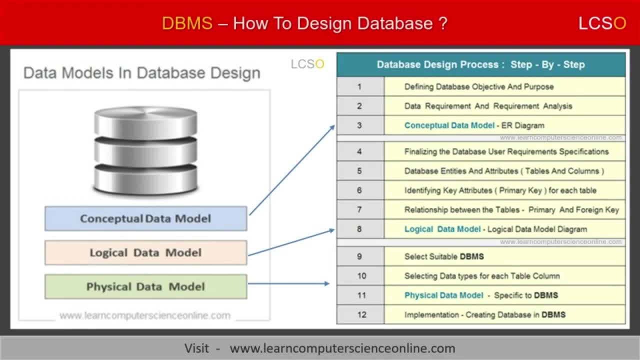 stages. The first step is the database planning stage, and the second step is the database building stage. Diese Organisation ist einen bestimmten, aunque großen Gesamtmodell, die says: die 두 z mới sonst anders gest. Let us dive into the details of the first stage. 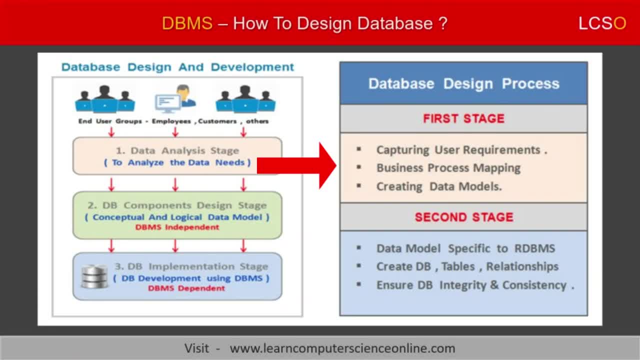 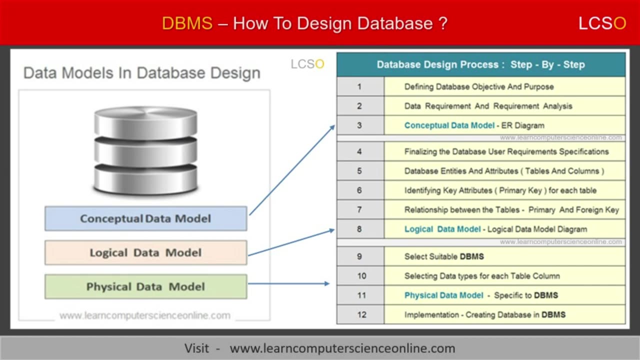 that is database planning stage snapshot. The first stage of the database design process is the database planning stage. This stage helps the design team to capture some valuable information that is crucial for the database design project. The planning stage is achieved with the help of creating two data models. 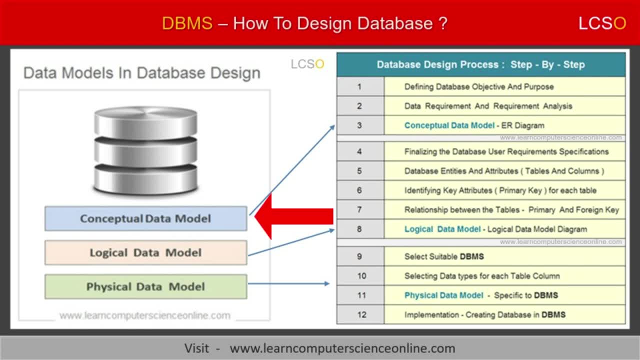 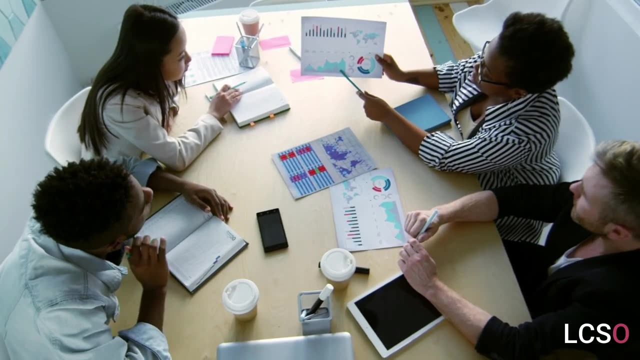 These two data models Are first the conceptual data model and second, the logical data model. The planning stage involve activities such as understanding the data requirements for various stakeholders and creating the necessary data models. At this stage, the design team also captures information about 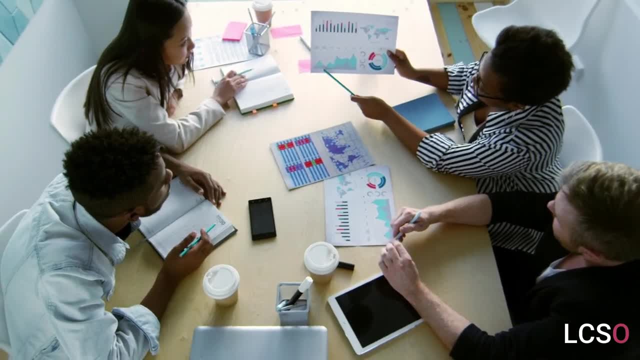 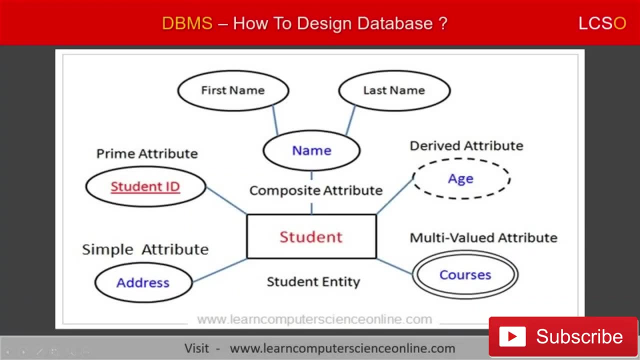 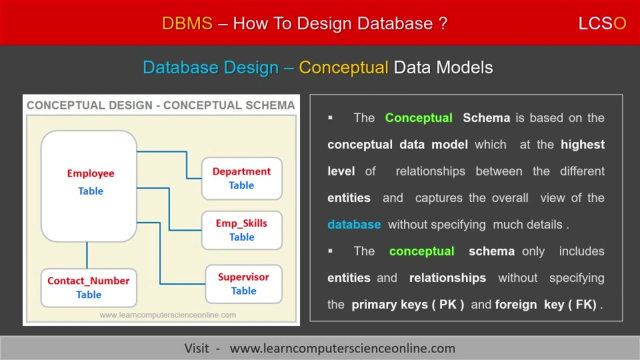 business operations policies, rules and procedures that the database should support. The entity relationship diagram ERD is an example of the conceptual data model constructed during the database planning stage. The conceptual database model describe the database view at the end user level with the help of simple diagrams. 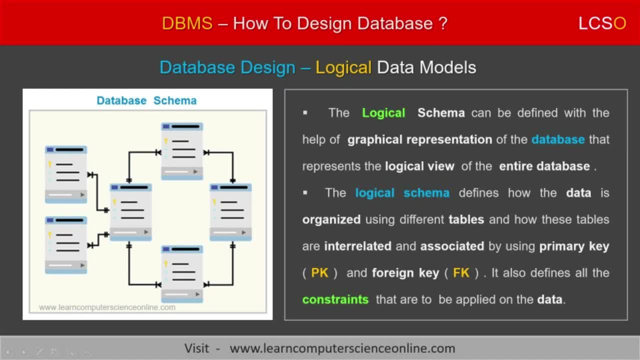 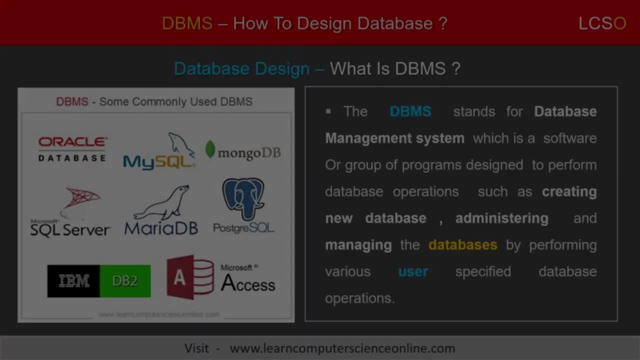 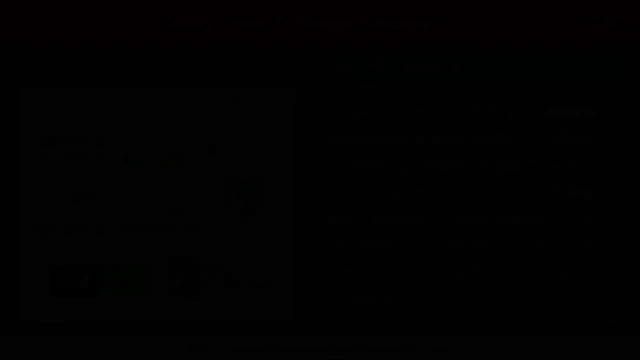 that are not DBMS dependent. The outcome of the database planning stage is the logical data model that can be implemented using any database management system, such as MySQL, Microsoft, SQL Server, Oracle or any other DBMS. During the planning stage. 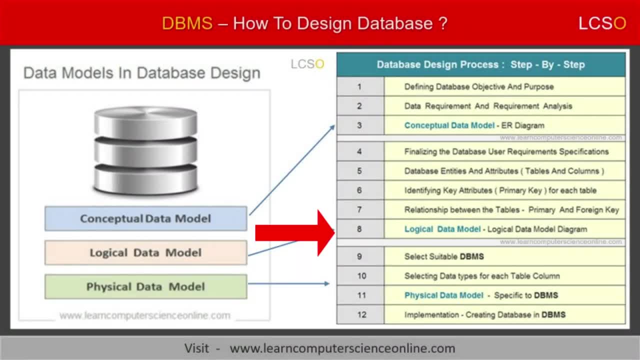 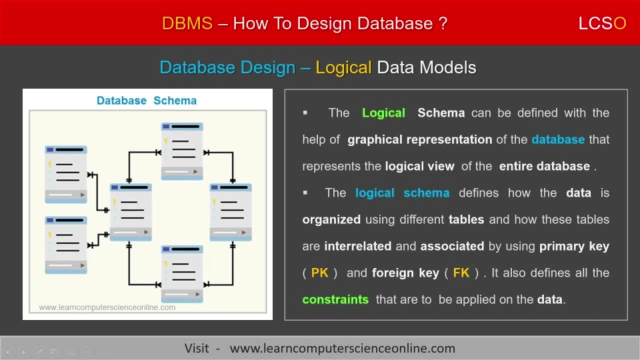 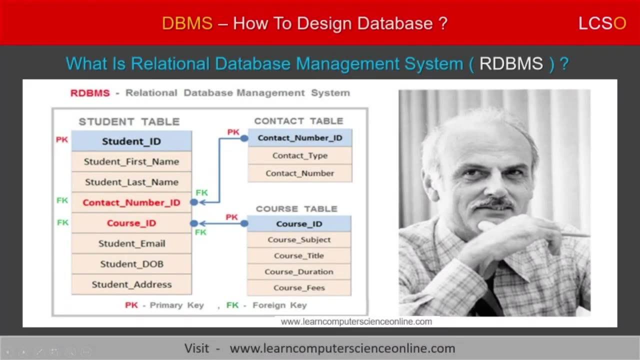 the logical data model is another important data model created based on the conceptual data model. The conceptual data model is further expanded to create a logical data model, For example for relational databases. the logical data model includes the details, such as database entities. 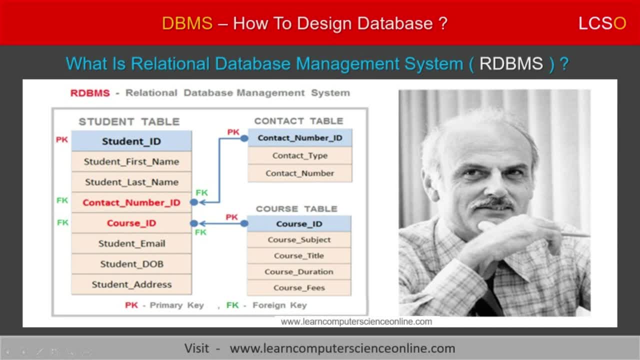 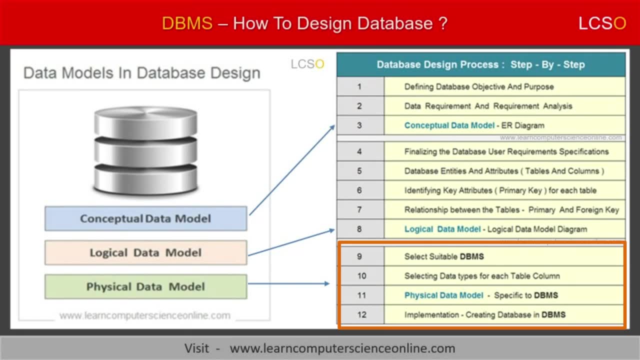 represented by the tables entity attributes, by the table columns and by defining the relationships between various database entities. The logical data model is another important data model. Let us now move on to the final stage of the database design and development project. 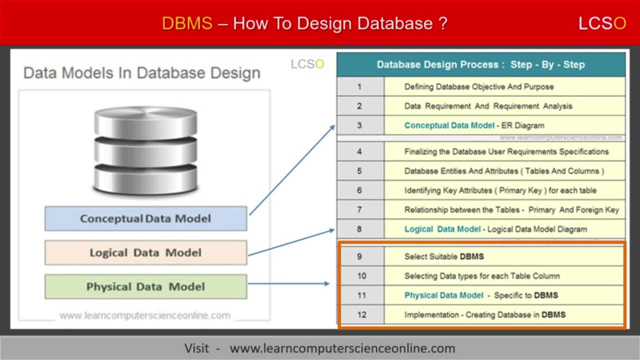 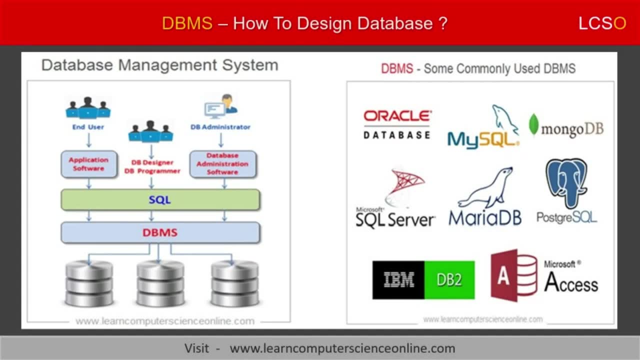 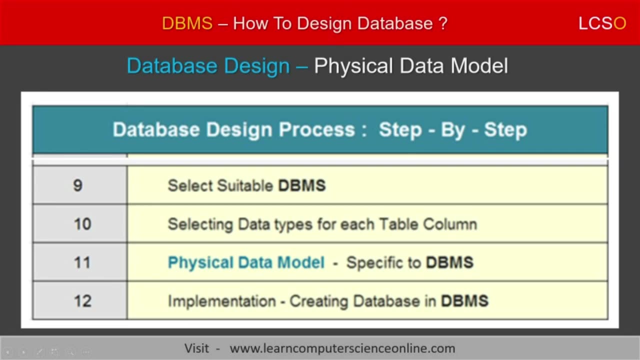 that is, building the database. After completing the planning stage, the final stage of the database design process involves building the database. The database is built using a specific database management system, abbreviated as DBMS. This stage is also referred as the implementation stage. In this stage, 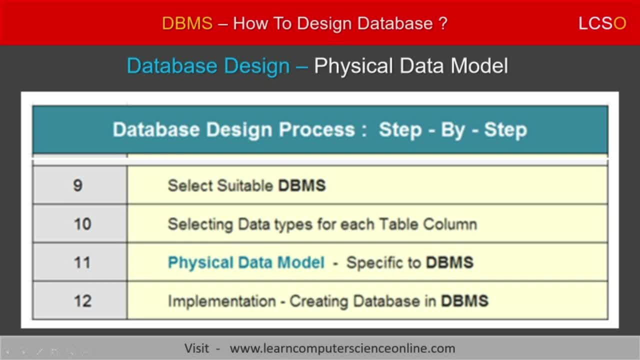 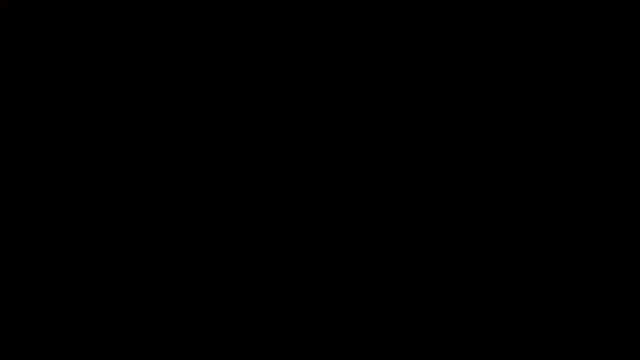 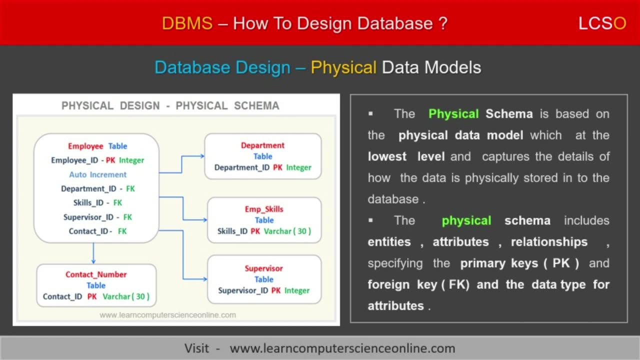 the database. designers build the database by implementing the physical data model. The physical data model is created by expanding the logical data model. It includes some additional details which are specific to the DBMS selected for building the database. The physical data model is DBMS dependent. 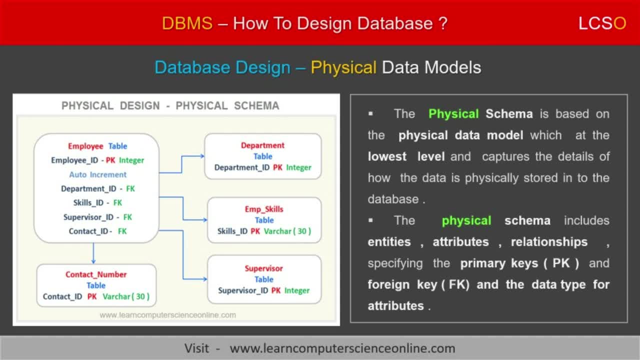 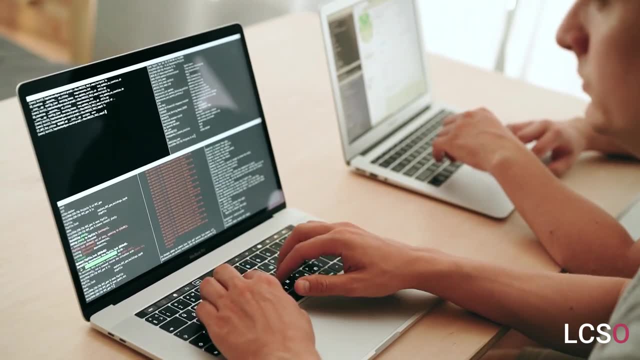 because it contains the details that can be implemented only on the specific DBMS. All right, as stated earlier, the database design process is specialist job and is a part of the database design process, And the design process is complex and quite elaborate. 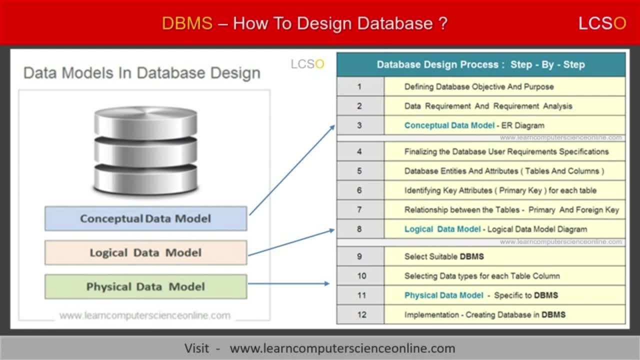 However, once you are familiar with the process, it becomes relatively easier to master each step of the database planning and design project. So this was just an overview of the entire process and subsequently we will be discussing each of these stage in detail. 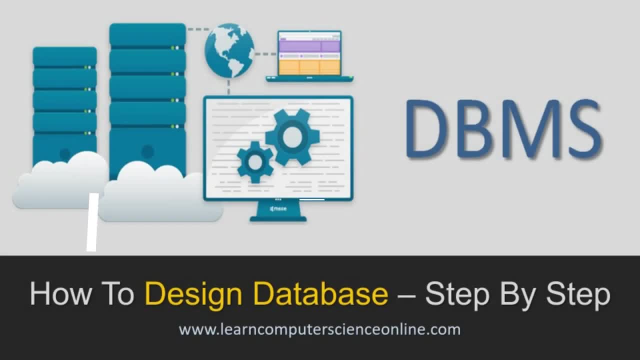 That brings us to the end of this tutorial. Please visit our website learncomputerscienceonlinecom to learn computer science online. If you have liked this video, then please give us a thumbs up and consider subscribing to this channel. Thanks for watching. and I will see you soon with another computer science tutorial.